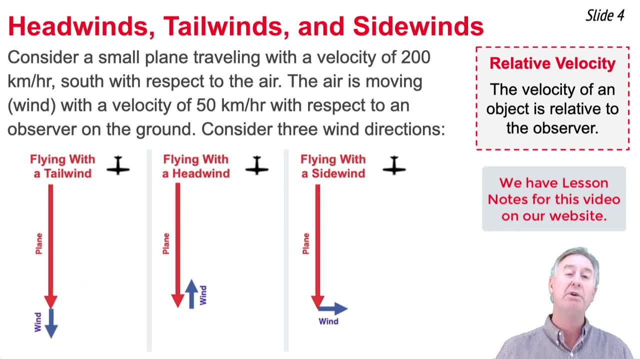 a tailwind. the wind is blowing the plane forward and the result is that an observer on the ground would observe a relative velocity from their reference frame of 250 kilometers per hour. in the middle there is a headwind. the plane is flying against the wind and because it is, 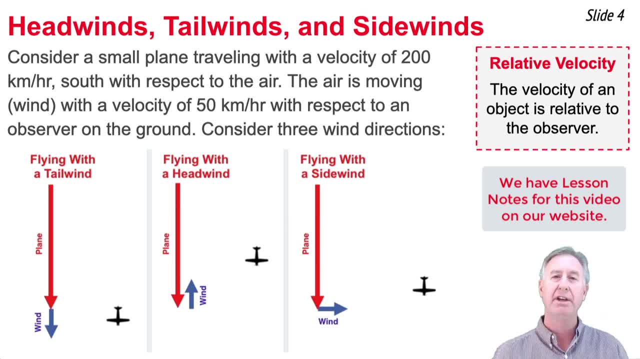 the velocity of the, as observed by an observer on the ground, is 150 kilometers per hour. in the case on the far right, what we notice is that the plane is flying with a side wind, and so pythagorean theorem would have to be used to determine the resultant velocity. as observed, 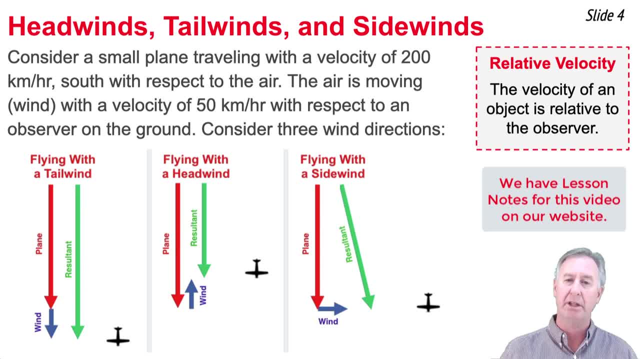 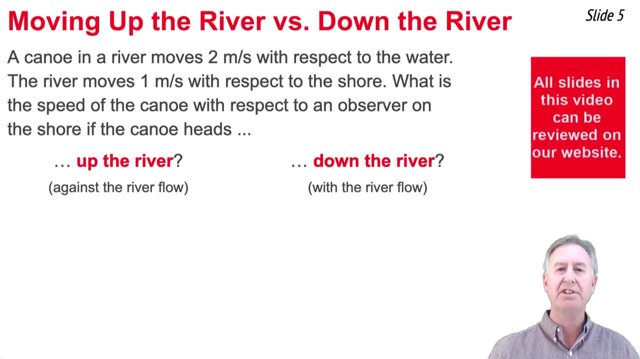 by that stationary observer on the ground, and it would be approximately 206 kilometers per hour. as another application of this idea- relative velocity- let's consider a canoe that can paddle at two meters per second with respect to the water, but it's river water, so it's moving and it's moving. 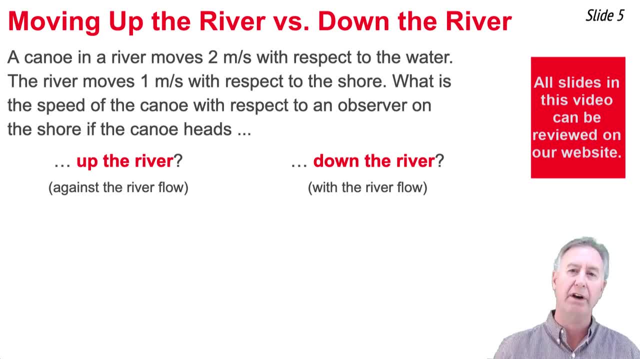 south at one meter per second with respect to an observer on the shore. and let's ask the question: what velocity would an observer on the shore observe of the boat traveling within this moving platform, the river? in the case of paddling up the river, what we would observe is that the boat 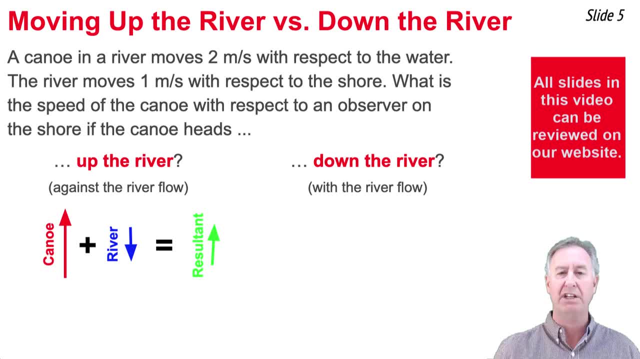 is paddling against the river flow, and so the river velocity subtracts from the boat velocity, and the resultant velocity is one meter per second north. and in the case of moving down the river, it's moving with the river flow, and so the river velocity adds to the boat's velocity and an 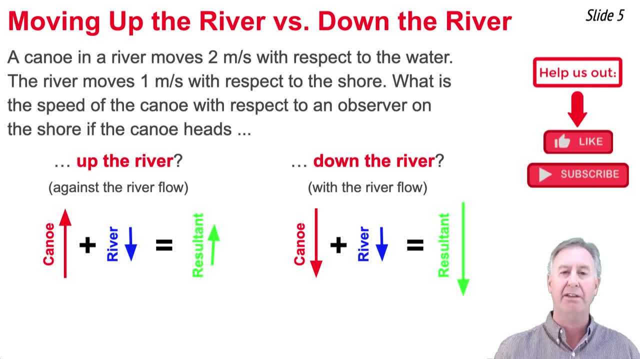 observer on the shore would observe a three meter per second velocity for the boat. in each of these cases, the observer on the shore is observing the resultant velocity of these two simultaneous, simultaneous velocities and it ends up being one meter per second north for paddling up the river. 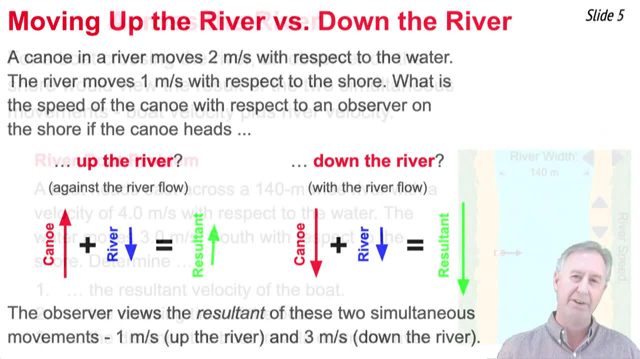 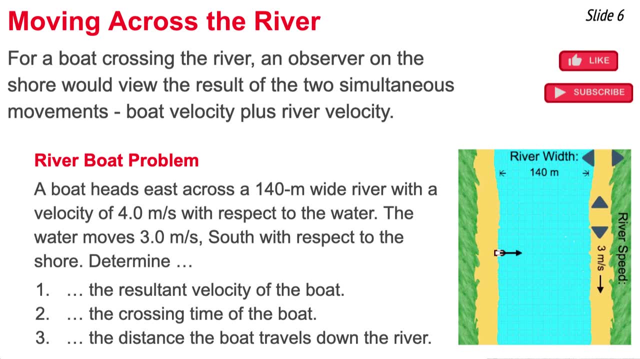 and three meters per second south when paddling down the river. now let's consider a boat that heads directly across a river, and the river is moving with respect to the shore, so an observer on the shore would re observe the resultant of these two simultaneous movements. a common problem is worded often like this: a boat heads east across a 140. 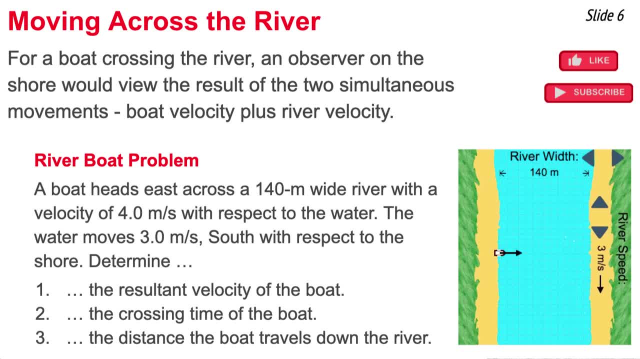 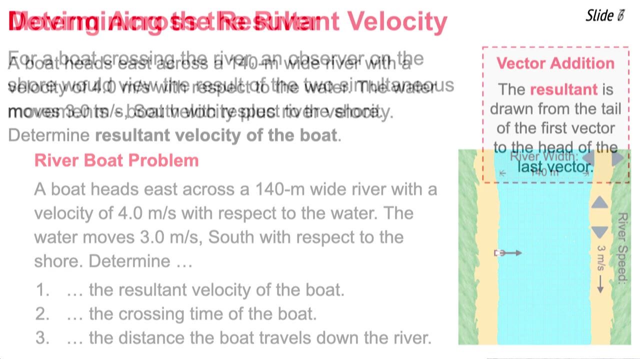 meter wide river with a velocity of four meters per second with respect to the water, and the water is moving three meters per second south with respect to the shore. 3 EFFECTS AND 3 QUESTIONS. question 0 0 0 0 0. 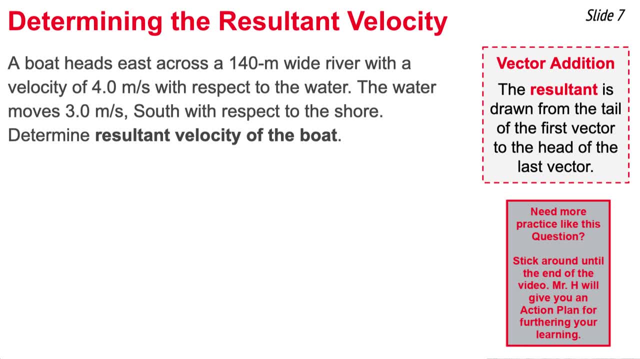 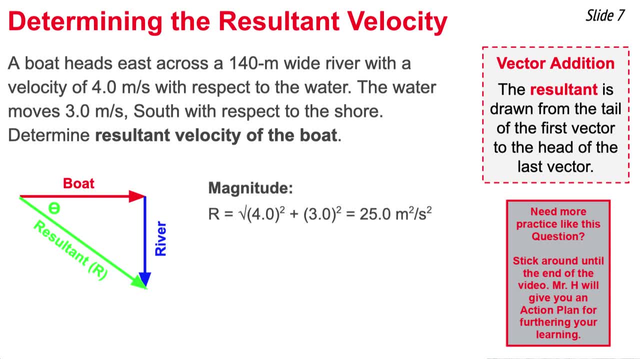 and its magnitude can be determined using Pythagorean theorem. So we say: r squared equals 3 squared plus 4 squared. Therefore, r is the square root of the whole thing. The square root of 25 is 5.0 meters per second. 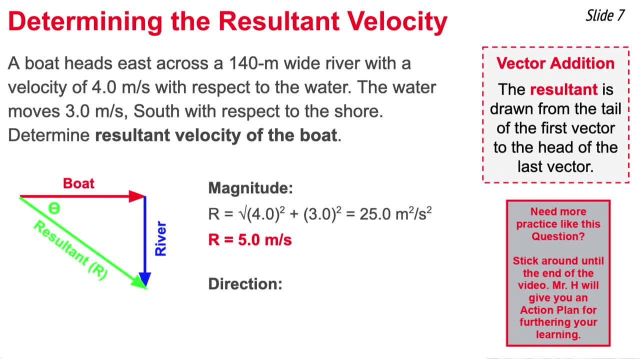 Now, to determine the direction of this resultant, we have to calculate the angle theta within that right triangle. The tangent of theta is the ratio of the side opposite, the river velocity, divided by the side adjacent, the boat velocity. That is to say, theta is equal to the inverse tangent of 3 divided by 4.. 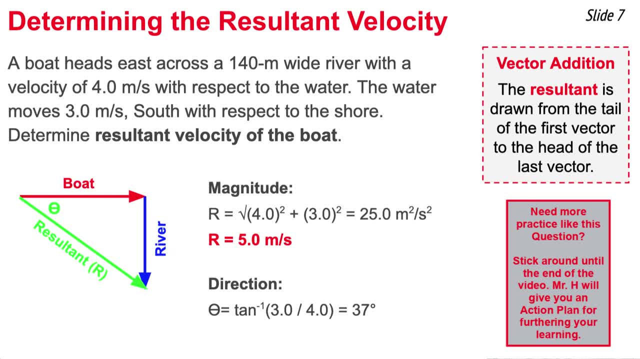 That comes out to be 37 degrees, the angle theta in the triangle. Now we have to express that as a direction. We have two choices. One of them is to say 37 degrees south of east And the other is to say that's 323 degrees wrapped around, beginning at east. 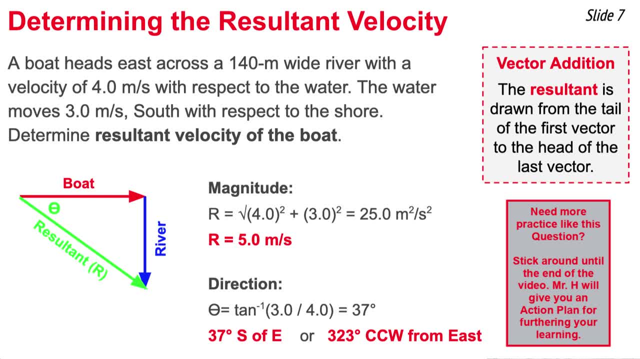 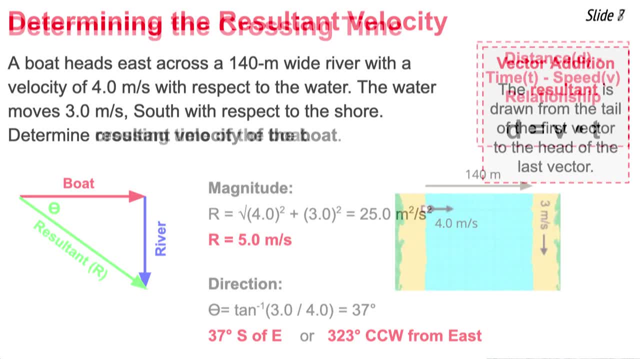 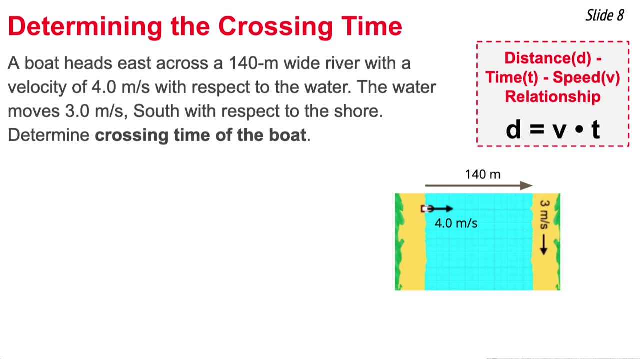 counterclockwise Past south and another 53 degrees past south, which gives us 323 degrees counterclockwise from east. The second question is to determine the crossing time of the boat, The time to go 140 meters from the west side of the river to the east side of the river. 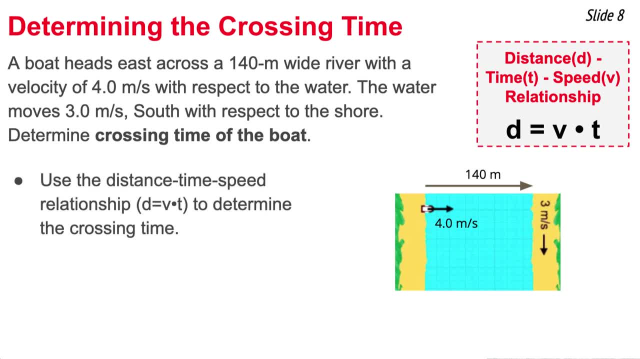 I can use the formula d equal v times t. It expresses a distance-time-velocity relationship. The only distance I know is 140 meters. I have to put that into the equation. But to solve for time I need to select the correct velocity. 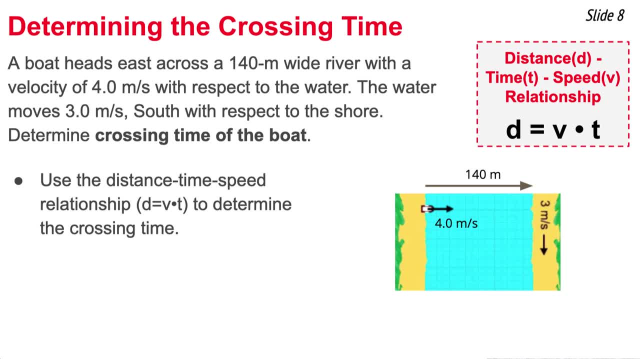 There's now three of them. There's a 4.0 meter per second east, a 3.0 meters per second south and a 5.0 meters per second, which we just calculated. that heads south and east, The velocity I wish to use. 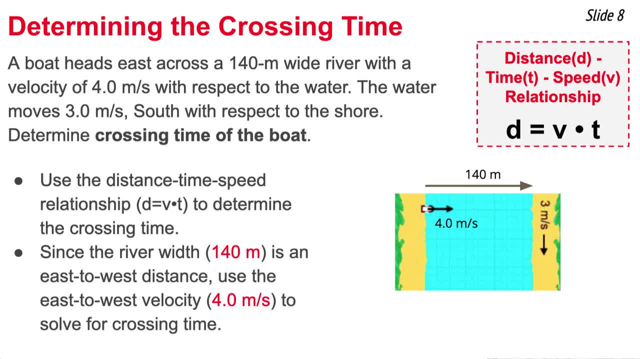 is the velocity of the boat traveling eastward across the river. Since I have an east to west distance, I need to use the velocity of the boat, to use an east to west velocity, And so I set up the equation to solve for time. 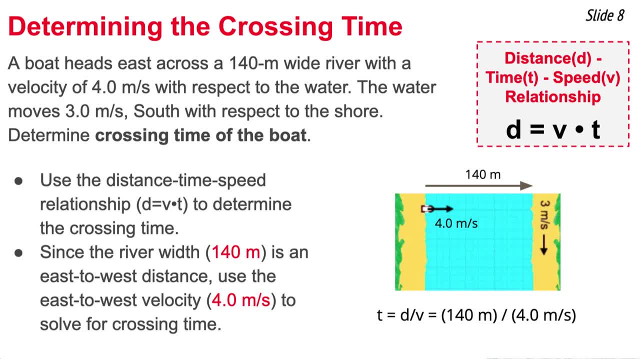 I say t equal d divided by v And I substitute 140 meters in for d and the eastern velocity of 4.0 meters per second for v, And I end up with 35 seconds, The final question of this three-step problem. 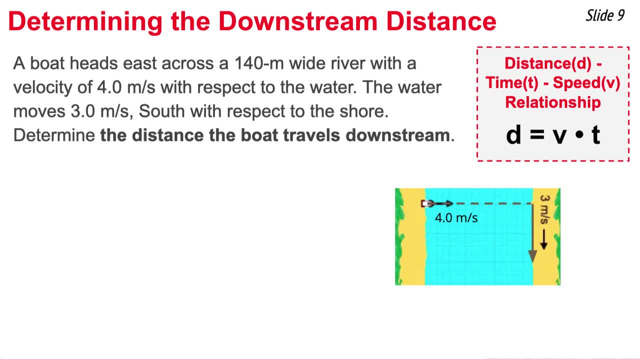 is to determine the distance that the boat travels downstream. So because it's a distance question, I need to use the distance and I'm going to use the distance equation. again, Distance is equal to velocity times time, And I want to calculate a downstream distance. 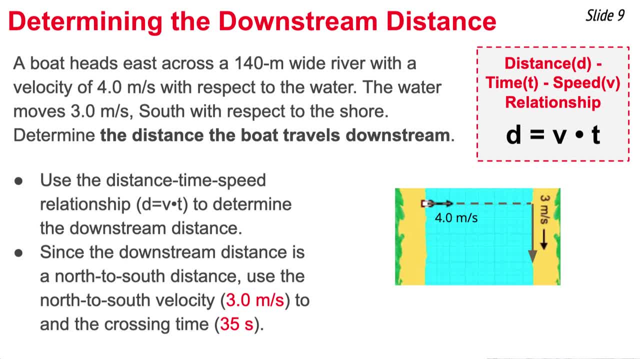 a down the river north to south distance, And because I do, I need a north to south velocity. It's this 3.0 meters per second that describes how fast I travel southward down the river, And so I have to combine that velocity with 35 seconds. 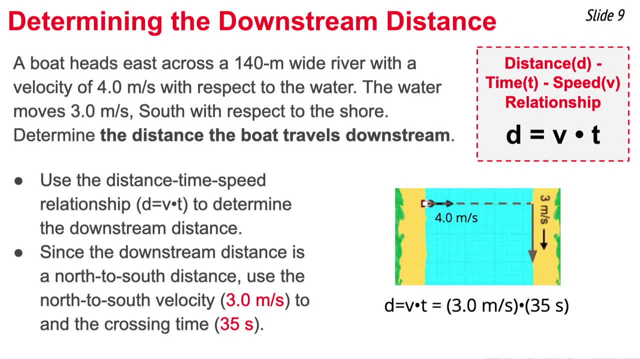 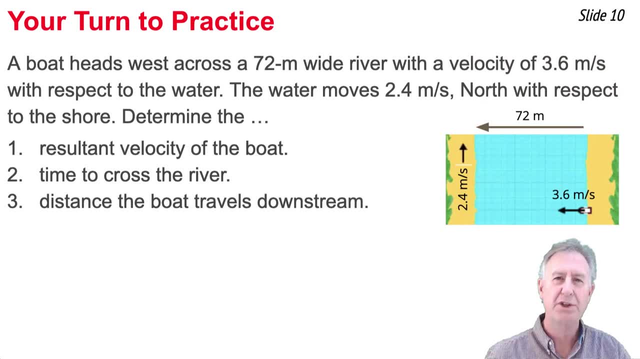 to determine the distance traveled downstream in the 35 seconds. When I do my math, I get 105 meters downstream. Now it's your turn to practice And practice with this problem here. So pause the video, read the problem, solve it. 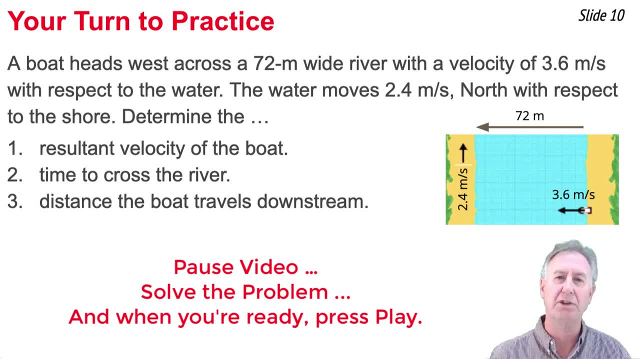 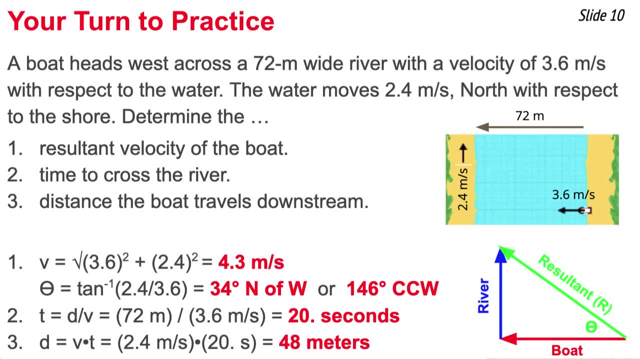 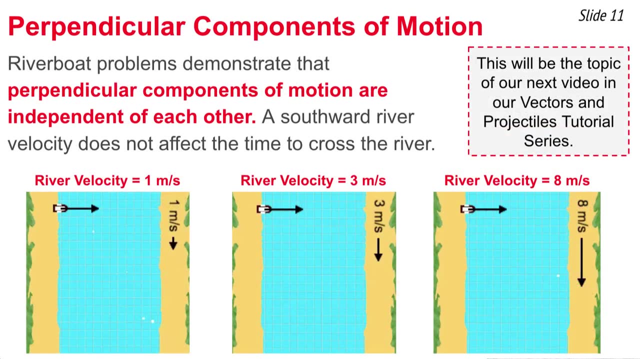 and, when you're ready, press play so that you can see the solution. And here is the solution. The concept that river boat problems teach us is that perpendicular components of motion are independent of each other, As you see here in these three animations. 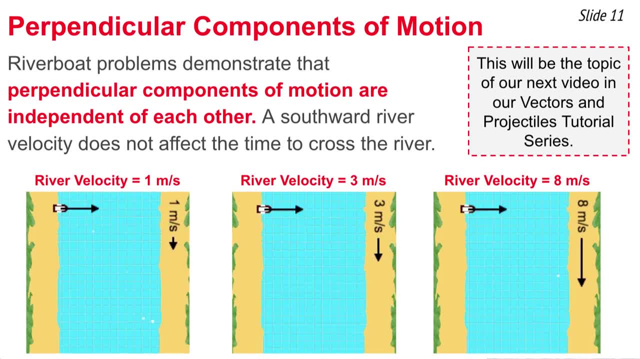 the river velocity is different, But the time to head east across the river is the same in every case. The platform on which the boat is traveling is heading south, But the boat heads east, And this southward velocity of the river